3 pm is going to be 1,500 hours, And then so forth until we get to midnight. Now midnight could either be 12.. 2,400 hours or 0-100 hours. Now, whenever it flips over to after we're getting past midnight, let's say 12.01,, 12.02, etc. etc. 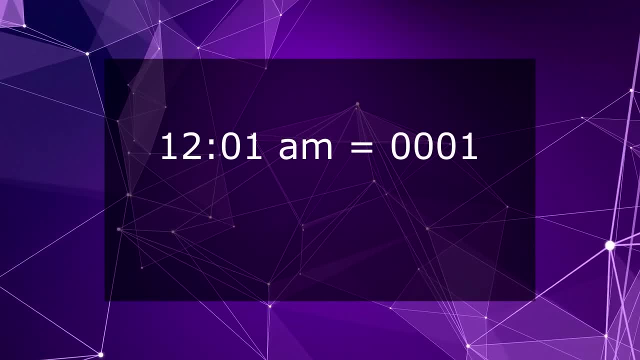 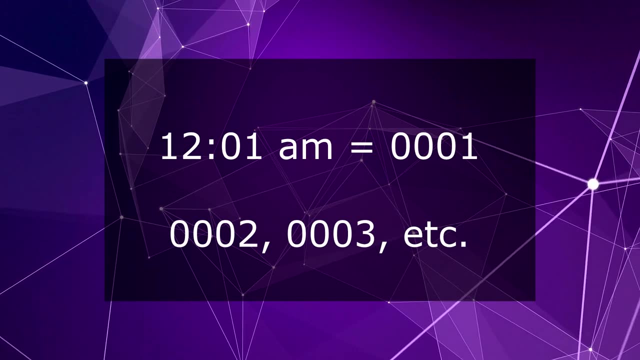 For 12.01, it would be 0-0-0-1.. And that time would keep going like that, such as 0-0-0-2, 0-0-0-3 hours, And there are different variations of how you can say these times. 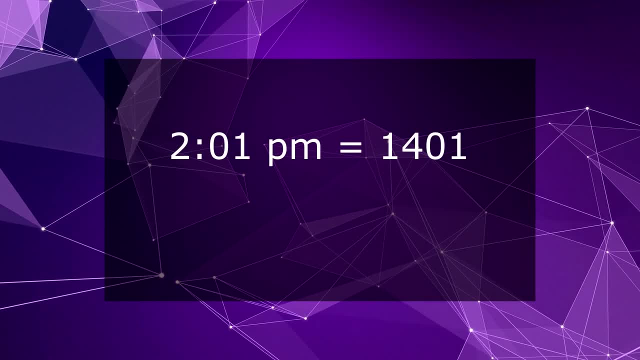 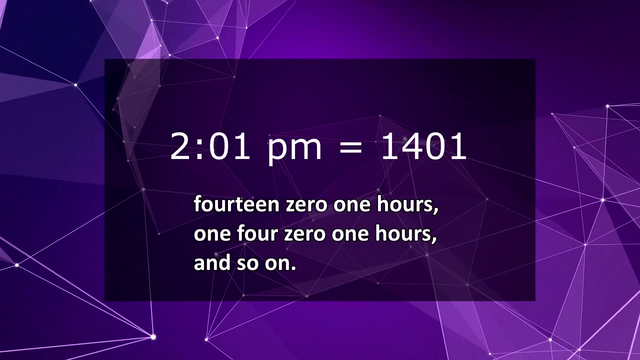 For example, 2.01 pm, which would be 14.01 hours, would be set as 14.01 hours, or 1-4-0-1 hours, and so on. Now, how can you remember these last 12 hours of the day? 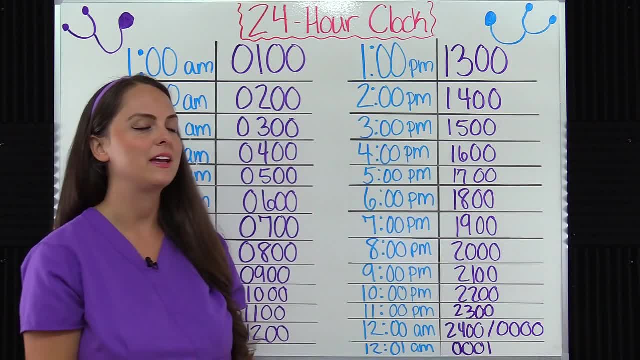 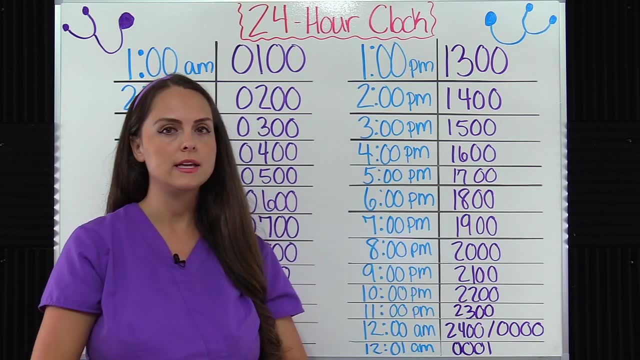 Because over here, the first 12 hours easy. Last 12 hours it takes some thinking. Well, remember the number 12.. So whenever we're trying to go from the 12-hour clock to the 24-hour clock- let's say it's 2 pm- all you have to do is add 12.. So 12 plus 2 is 14.. 3 plus 12 is 15.. You got your time. Now let's say you're in military time, but you're trying to get back to the 12-hour clock. You subtract 12.. 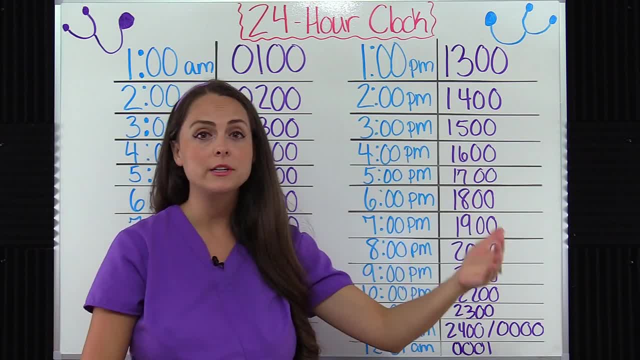 So if it's- you see the time- It's 14.00, subtract 12, you're going to get 2.. So you know it's 2 pm. If it's 15.00, subtract 12, you get 3.. 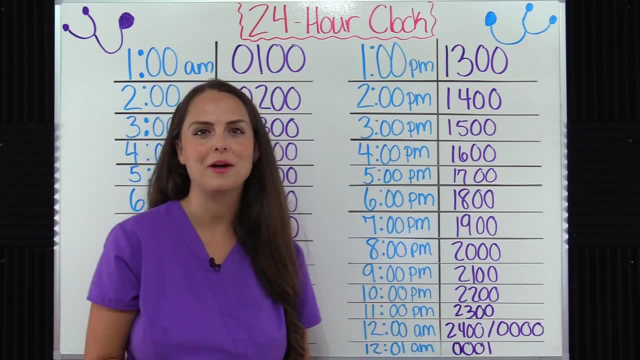 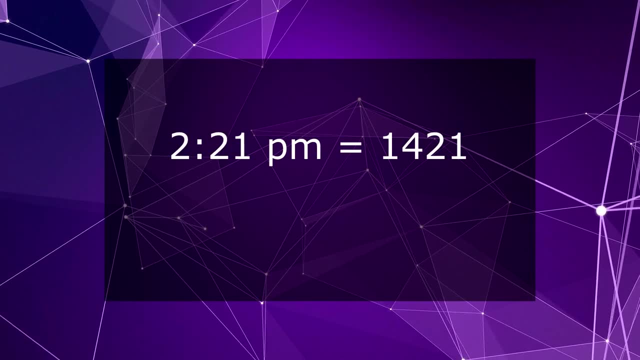 You know it's 3 pm, So hopefully that little trick will help you Also. let me give you an example of military time with minutes. How would you say that? Well, let's say the time is 2.21 pm. 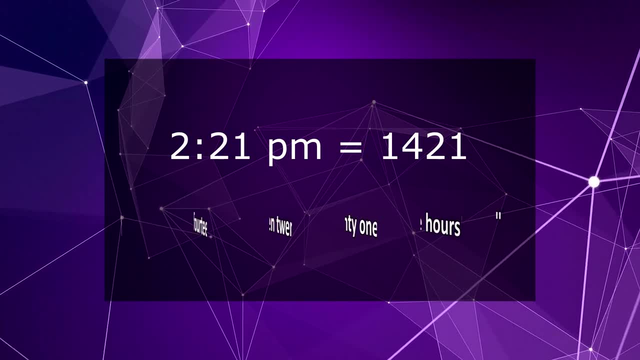 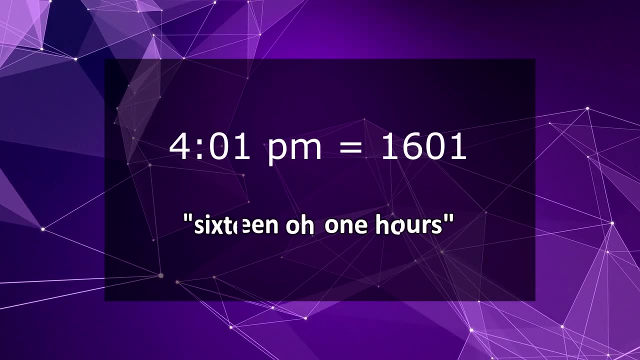 so 14.21.. How would you say that You would say it as 14.21 hours? And another example would be, let's say, 4.01 pm. How would you say that You would say that as 16.01 hours? 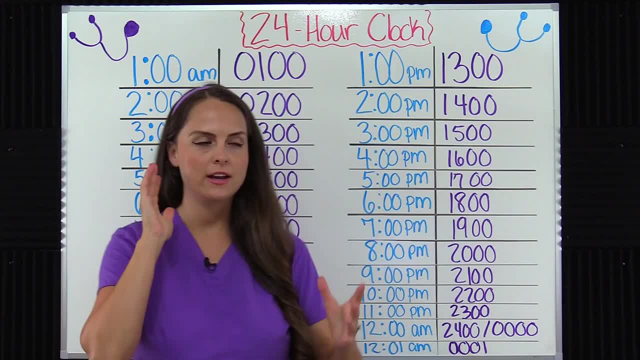 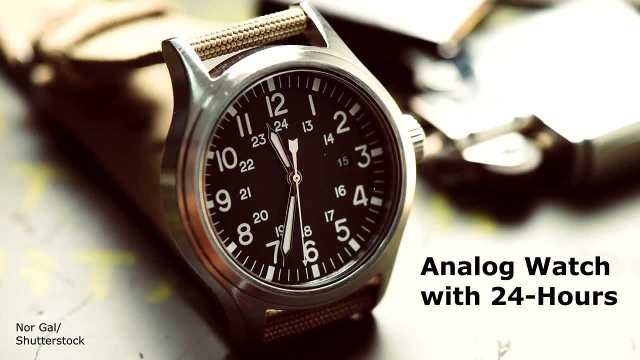 Now, let's say you cannot get this information to stick in your head. It's just too confusing for you, going between 24 hours to 12 hours. Well, whenever you're first starting out as a nurse, what you can do to help yourself out is you can get a watch. 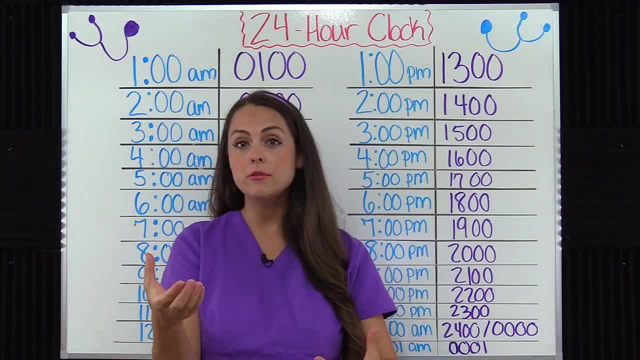 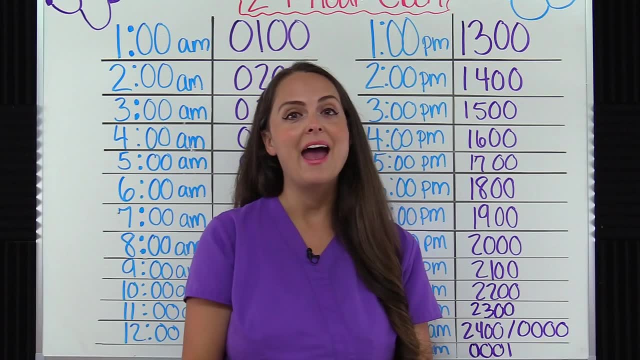 and put it in military time, Or you can set your phone to that as well, or maybe even the computer that you're using at work. you can set that to the 24-hour clock, But after a while, once you are doing this day in and day out.